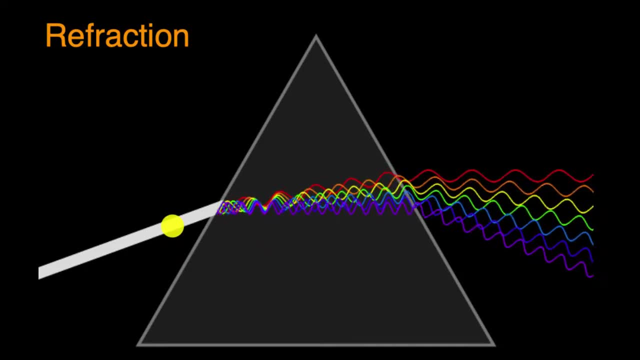 This process of when light goes from one transparent medium to another or a vacuum to some other medium that it can travel through, that's transparent. if it hits it at an angle, it can get bent, which is what we call refraction. This is why, when you look at a cup of water, 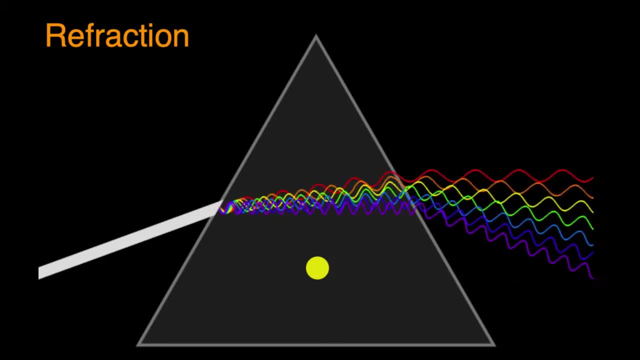 or at a pool at an angle you're not seeing directly through the pool, The image gets distorted. 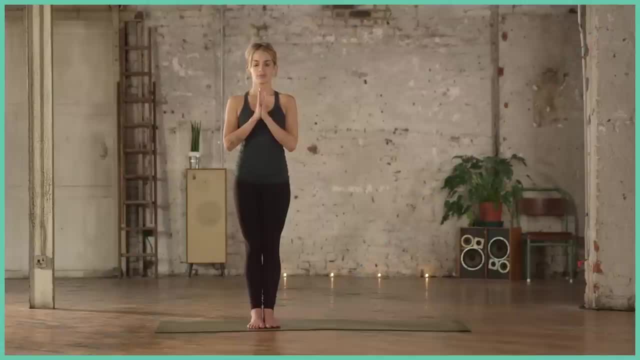 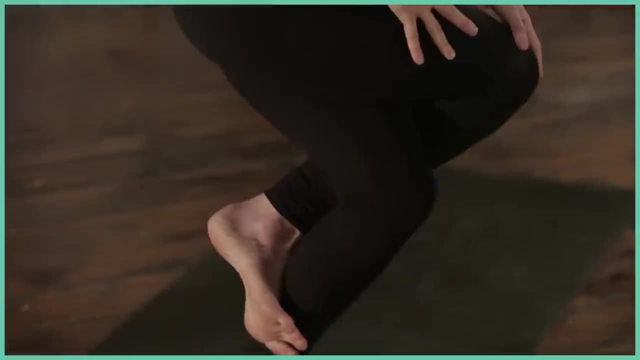 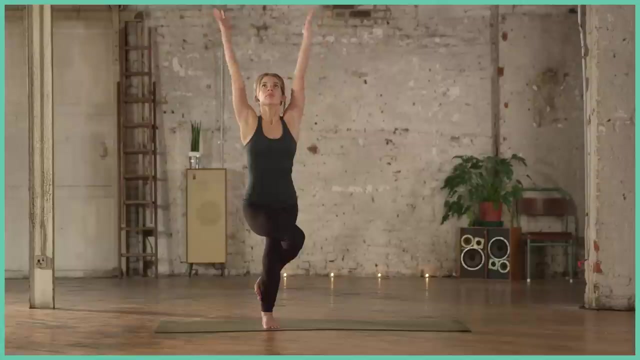 Starting with the hands at the heart center. From here- inhale, lift the knee into the chest, slowly wrapping that right leg around the left. Maybe it goes once, just like that, or maybe it wraps twice. From here- inhale, sweep the arms, press the palms, Exhale. 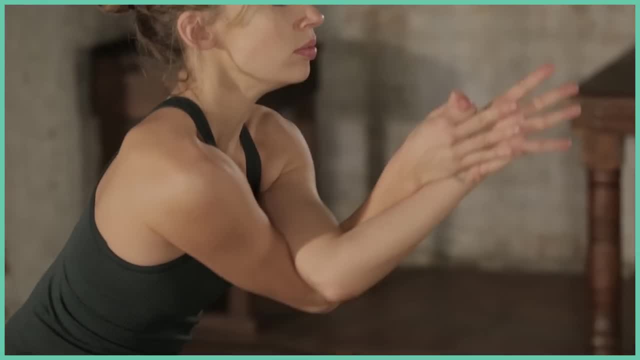 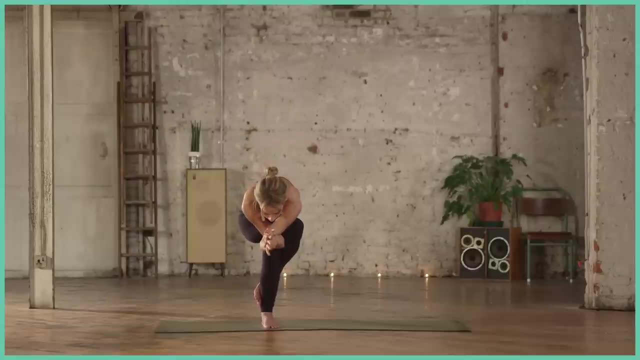 right arm underneath. Inhale, lift the elbows away from the chest. Exhale- you can stay here with a straight spine. Otherwise, bring the elbows to the knee, coming into full eagle pose, Breathing in, breathing out, finding balance From here. inhale, lifting up, bring that knee. 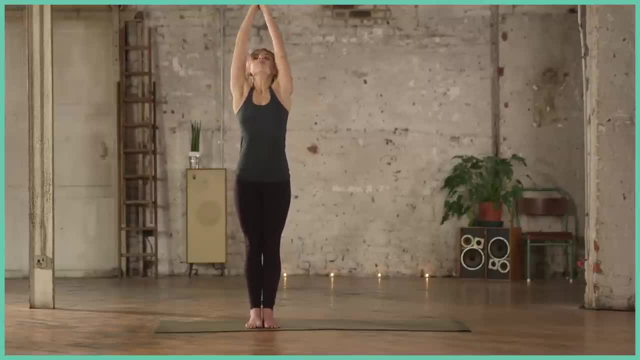 back into the chest. Exhale release Hands to heart, center On the left. now, From here, inhale left knee into the chest Again, guiding that leg around the standing leg. maybe once, maybe twice. From here, inhale sweep the palms, press to touch Exhale left arm underneath this time. 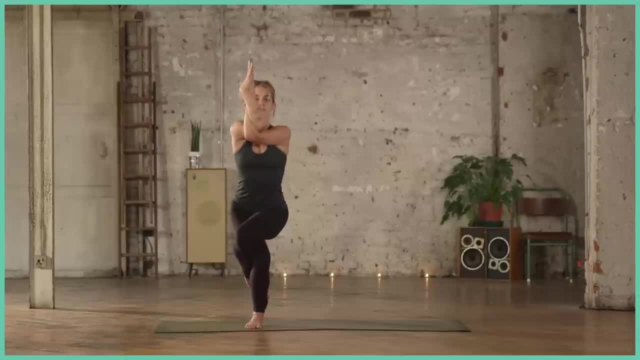 Inhale, elbows away from chest, create that space. From here you can go all the way or stay up nice and tall, Breathing in, breathing out, finding your balance, staying strong. Inhale, come all the way up, unravel, press palms to touch. 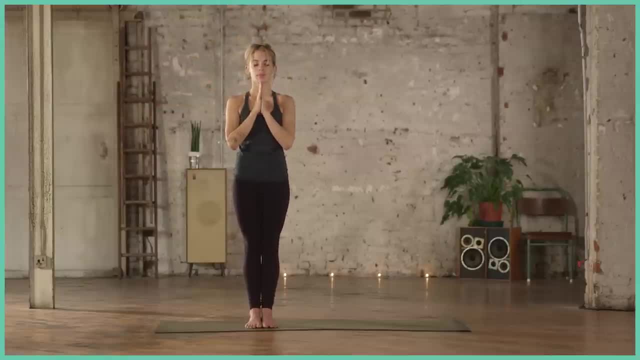 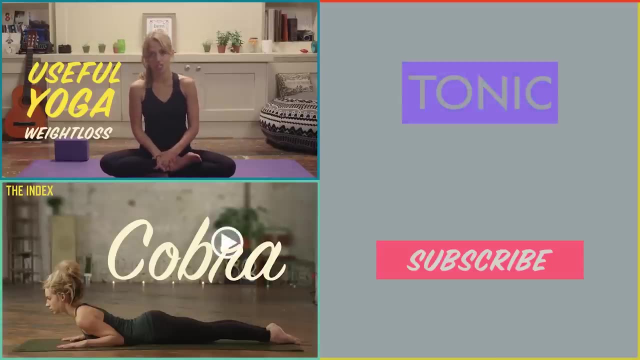 Exhale release back to standing. Today's session is all about weight loss, So sometimes yoga gets a bad rep for being easy and boring and slow. Well, this class is going to get you sweating. It's going to get you burning those.